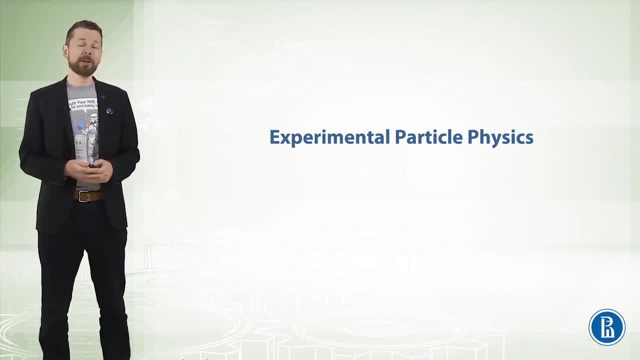 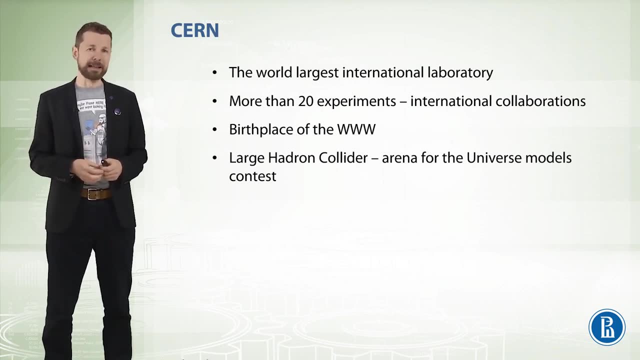 predictions for further experiments. CERN is a French abbreviation for ¡Ñ CENTER OF EUROPEAN NUCLEAR RESEARCH. Essentially, it is a vast laboratory. There are several distinct experiments that take place, and everyone is operated by an international collaboration that unites physicist or 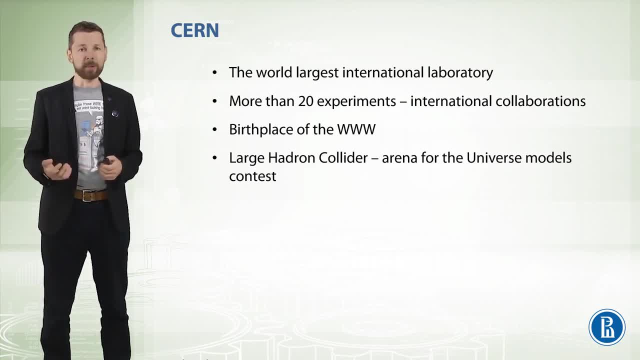 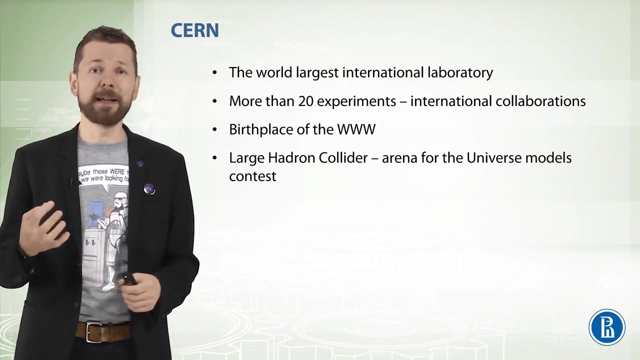 scientist from different countries, People from hundred different countries work together and carry out the- together, despite political difficulties and misunderstanding on governmental levels. They focused their intellectual efforts on the development of better understanding of our universe, on the development of new technologies. So it is a fascinating place and there are, of course, some byproducts that you are most. 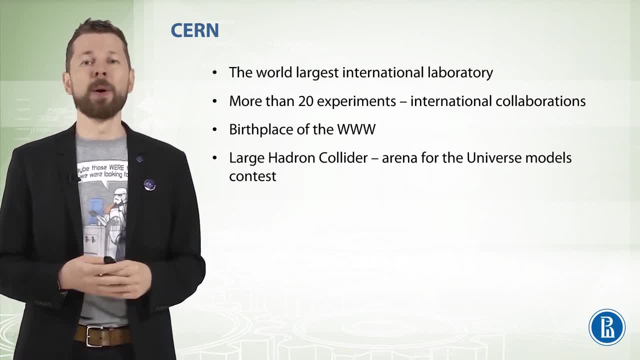 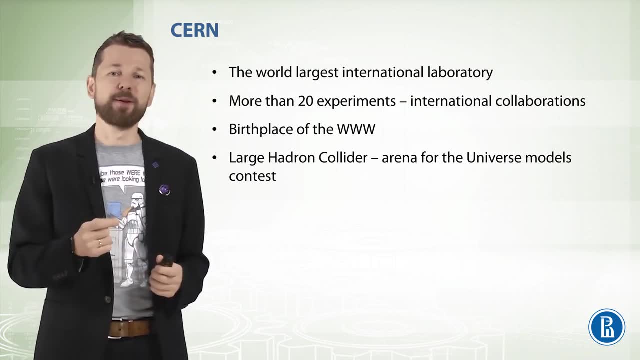 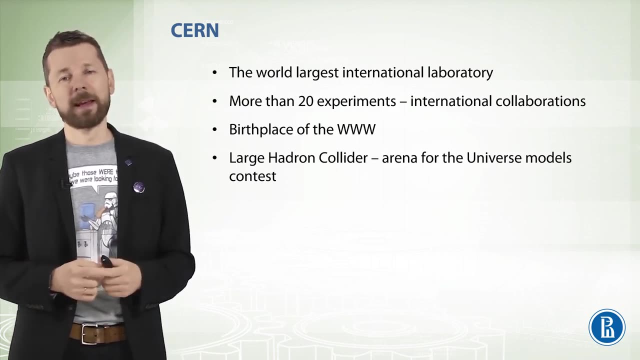 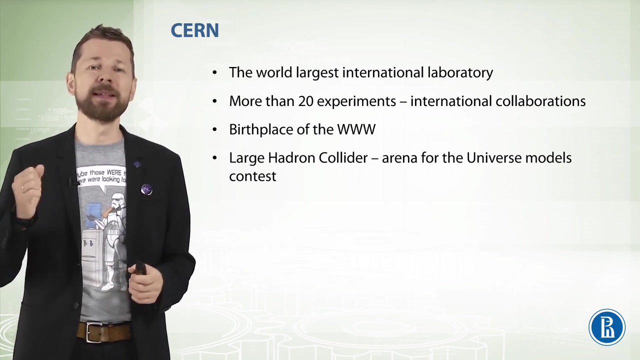 likely aware of, For example, CERN is a birthplace of the World Wide Web, So you are using this to watch this lecture. Also, one of the great things built there is called Large Hadron Collider. It has been used for discovery of Higgs boson and it is one of the finest and the biggest. 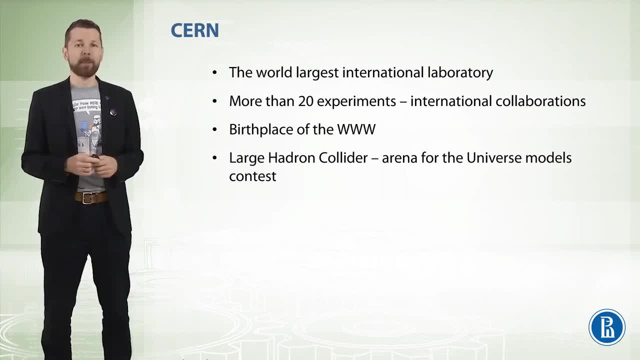 data generation machine ever created. By design, it is a machine for smashing protons And examining outcomes. By the fact, it is a massive arena for examining different models, striving for better explanation of the universe. Let us take a closer look at LHC. 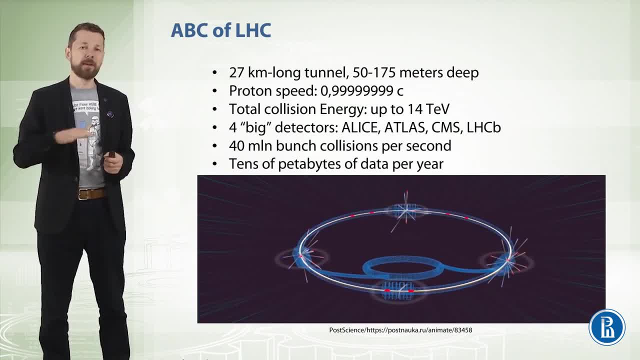 It is a 27 km long tunnel, 50 to 175 m deep, and the protons are accelerated to the speed almost comparable to speed of light. The speed of light and the energy collision of those protons is up to 14 teraelectron volts. 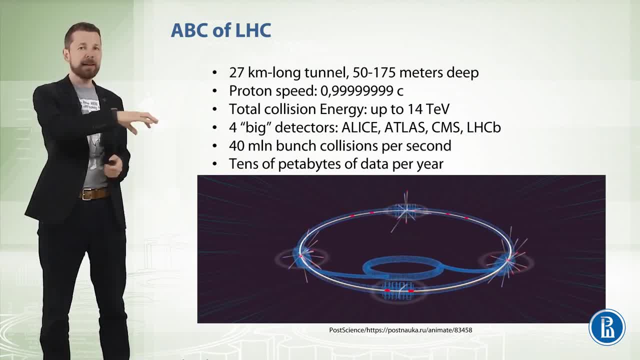 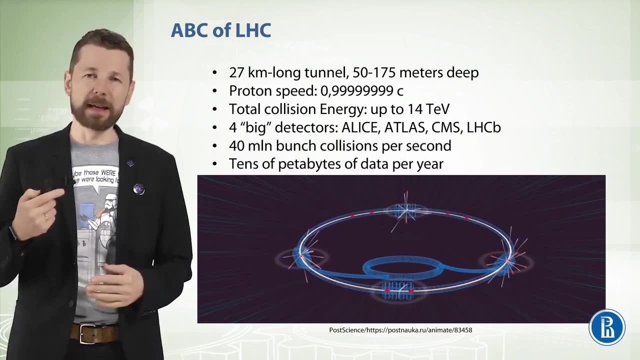 There are four big detectors located around the ring. Those are called ALICE, ATLAS, CMS and LHCb. So there are 40 million bunches of protons that collide every second. Every detector generates enormous amount of light. It is a very large amount of data. 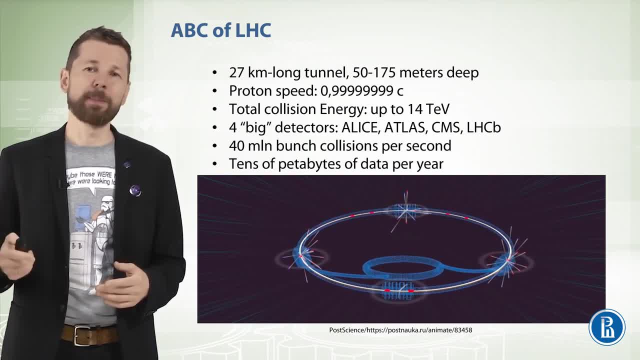 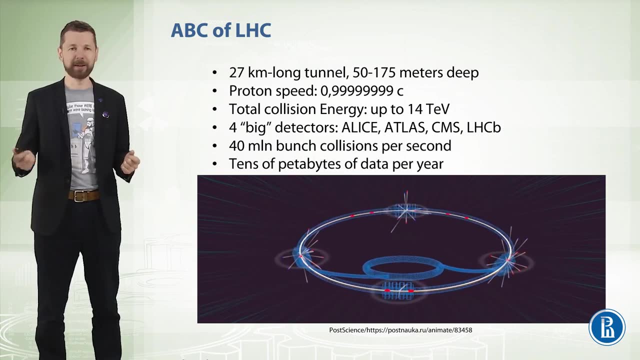 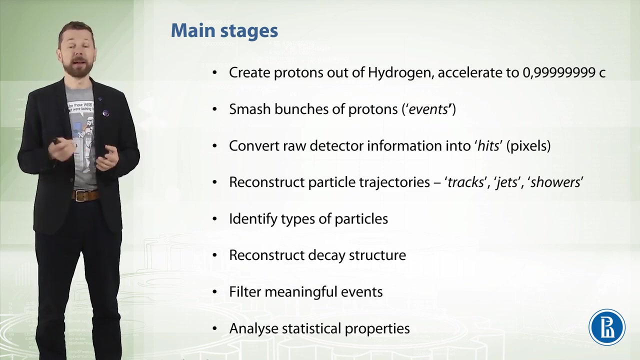 For example, since the beginning, hundreds of petabytes has been stored for later data analysis. Let's take a look at the cycle that starts from the very beginning till the discovery or publication has been created. So we start with creation of protons out of hydrogen atoms. 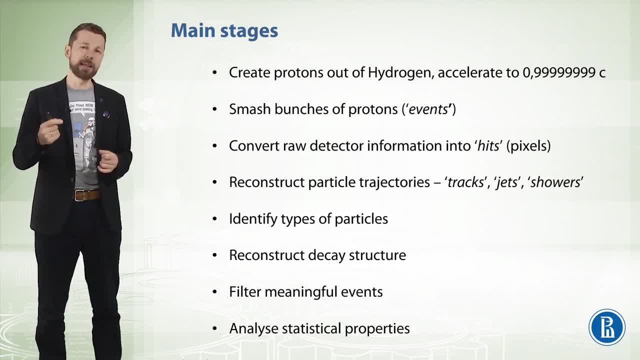 And then we accelerate those To the speed almost equal to the speed of light. Then those protons are grouped into bunches. Those bunches are smashed into each other and during this collision, set of particles appear out of the energy of this collision. 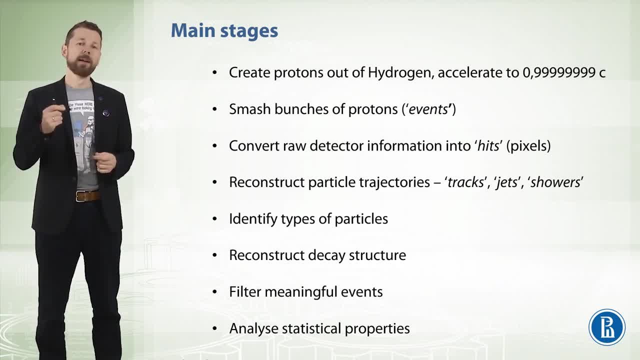 Those are called events. Then the detector that sits around place of this collision, This detector is called a fusion, It is called a fusion. This is a fusion, This is a fusion, This is a fusion, Then this is a fusion, Then this is a fusion. 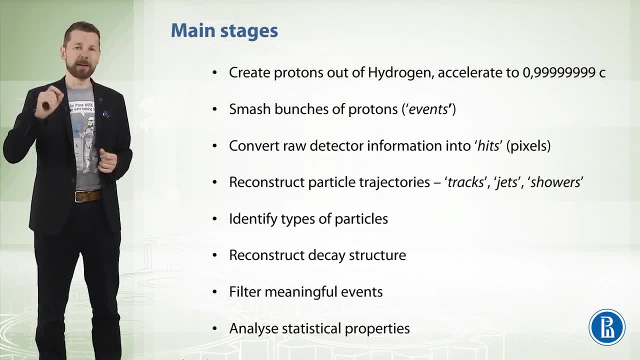 It records information of the energy that is deposited by every particle flying out of the event and converts this information of the energy into the hits that you can record and store. After this, the algorithm that tries to reconstruct trajectories of different particles and identify types of those particles comes to action. 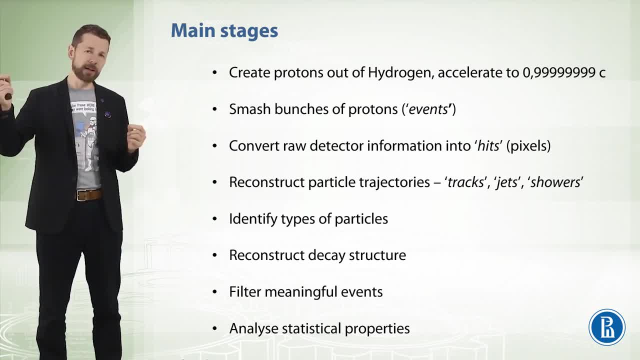 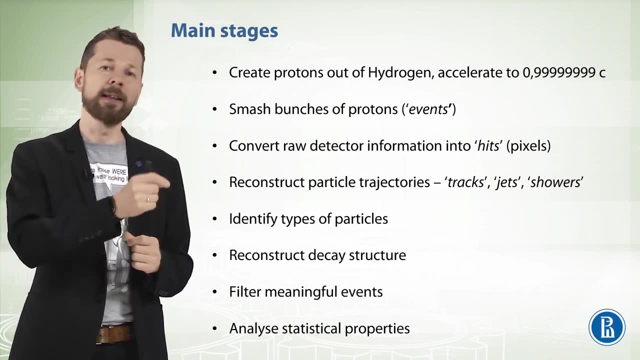 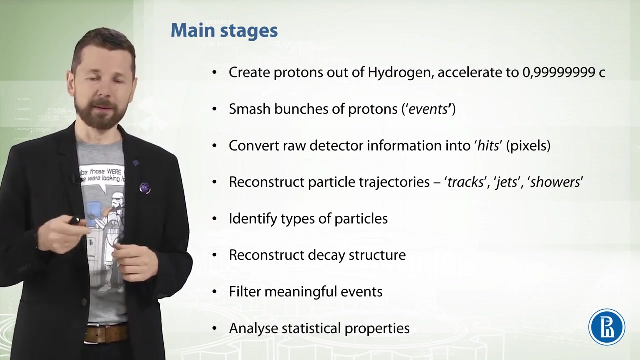 After we get a picture of individual trajectories, we combine them into vertices and form a structure of the whole event. Then we build a map of the event and filter for the further analysis only those that have some meaning from the physical point of view. And only after this we analyze statistical properties of those events that have been stored. 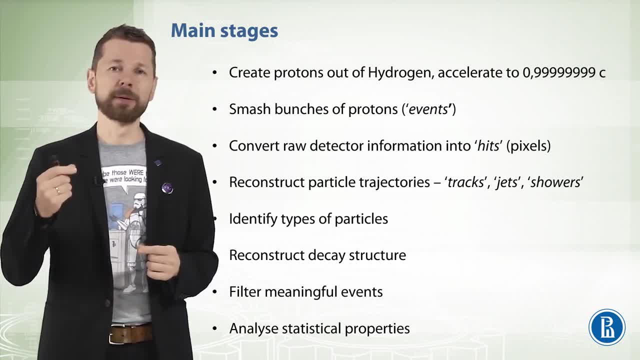 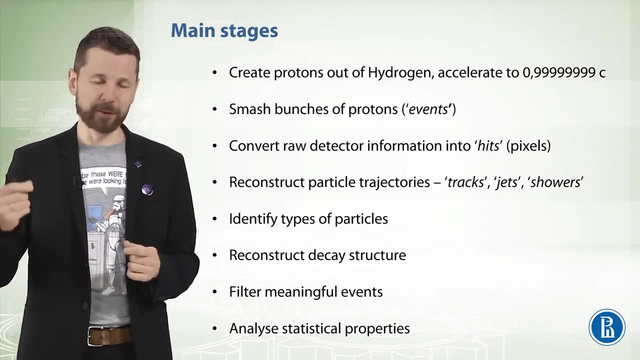 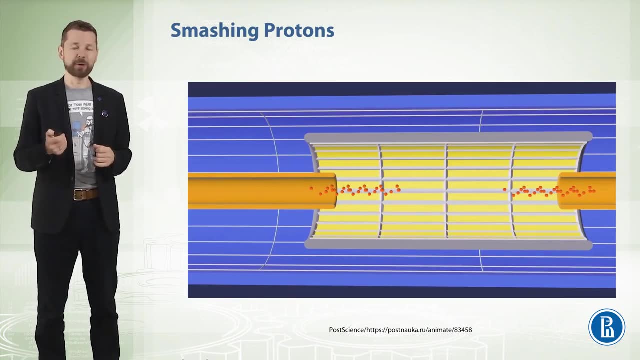 and make conclusions about the validity of models that predict the existence of certain parts of the events. Let's take a closer look at the stages that happen during the data collection. So here you see a schematic image of the detector and two bunches of protons flying to each other. 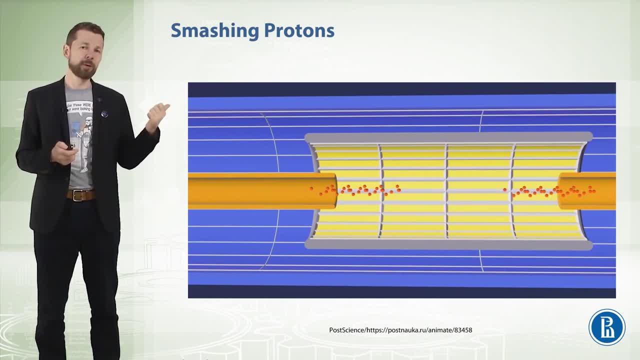 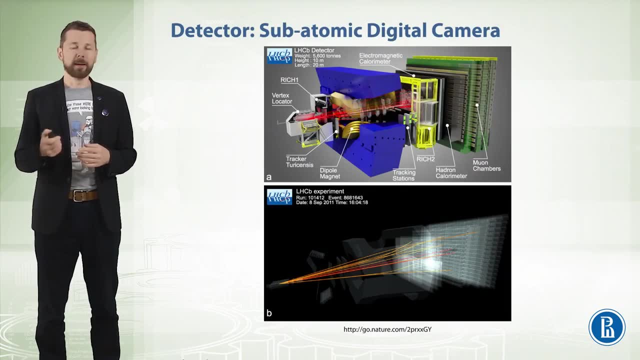 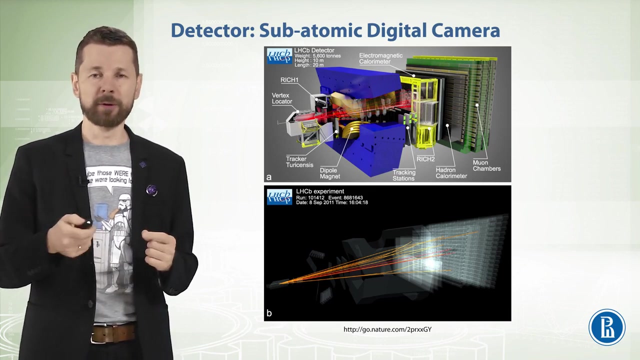 There is actually a movie that you can look at if you follow the link below. that describes this process a little bit nicer. So at the place of collision there is a detector, which is essentially a subatomic digital camera that sees and records outcome of the collision that happens during the data taking. 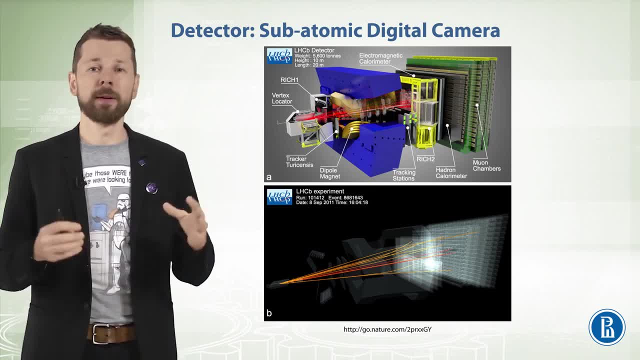 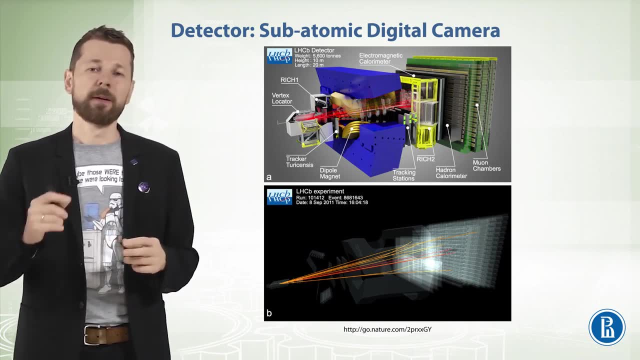 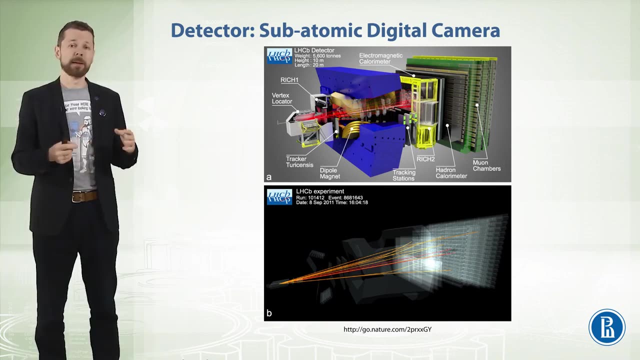 On the upper part of this image you see the mechanical design of LHCb detector and at the bottom part of this image you see reconstructed trajectories of elementary particles that has been detected by this detector. So at the right part of the image, of the bottom image, 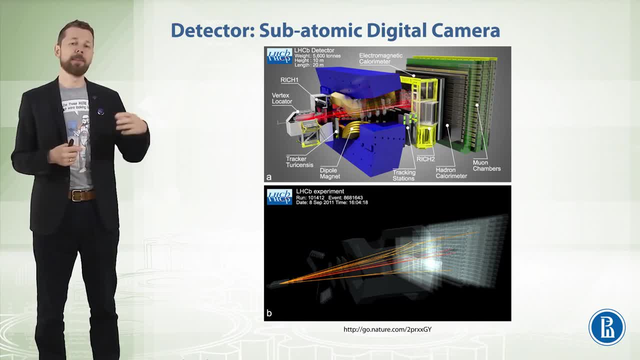 you see schematic grids that represent sensitive part of the detector and there are colorful lines that has been reconstructed from the data collected from those grids. So here is a close-up look at those part of the detector. You see green and blue rectangles that represent hits of the particles that has been recorded by the sensitive element. 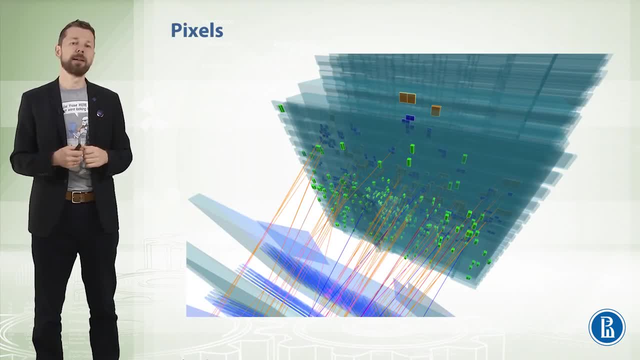 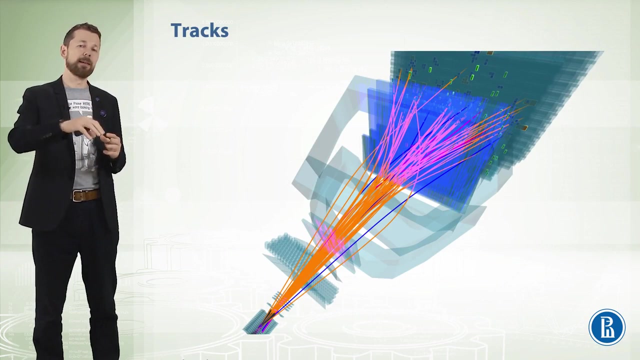 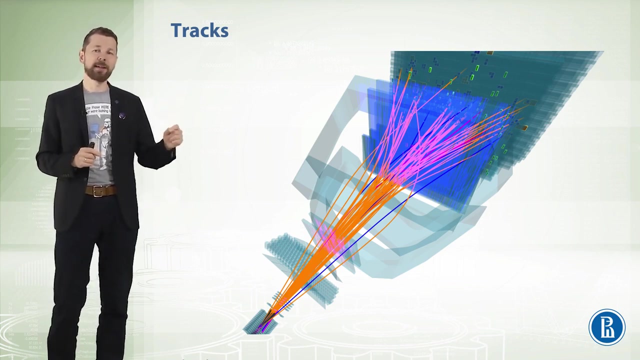 and those hits actually produced by particles, and we can reconstruct parameters of trajectories that created those hits. So the colorful lines are exactly those lines. So here you see the collection of lines that has been reconstructed for the whole event, and the data is used for this analysis, for this reconstruction. 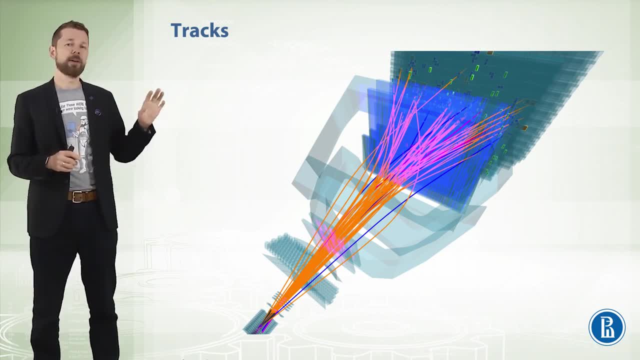 come from various parts of the detector. It's not only the back side or downstream side, It also comes from. there is a middle part that is called tracker, and there is a very precise part of the detector that sits around the place of the collision. 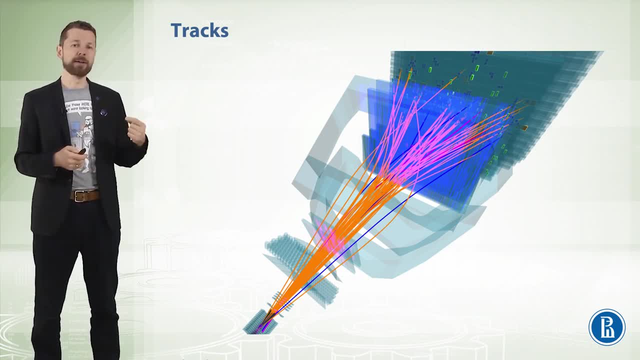 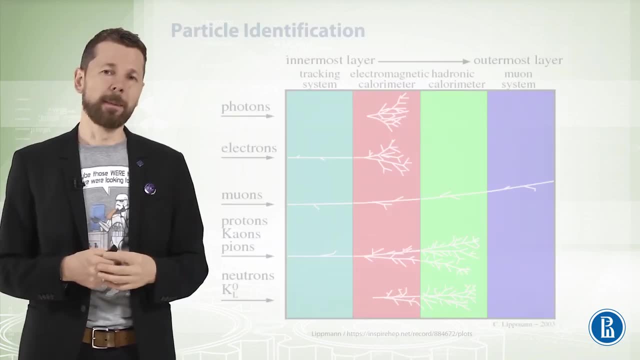 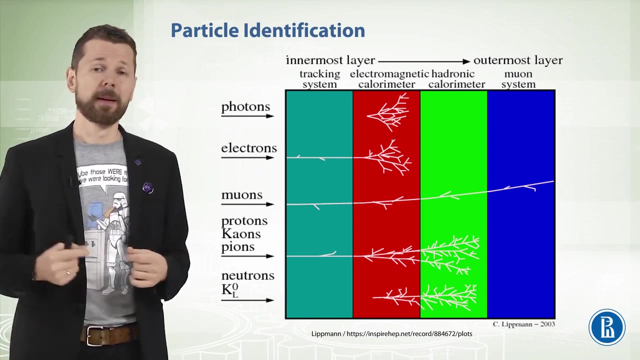 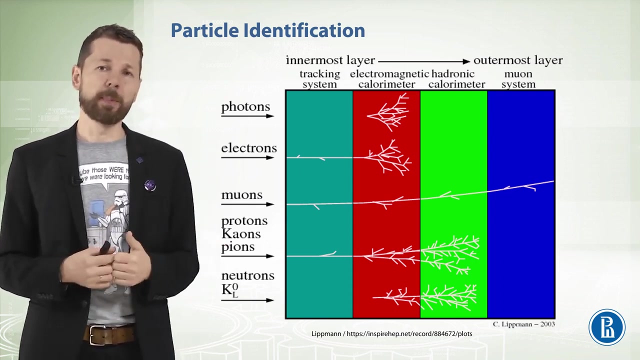 It is called vertex locator. that creates gives most of the information about the particle trajectory, And then we have to identify what kind of particle every track represents. We can use various sources of information. The first one is that every particle leaves different traces in different sub-detectors. 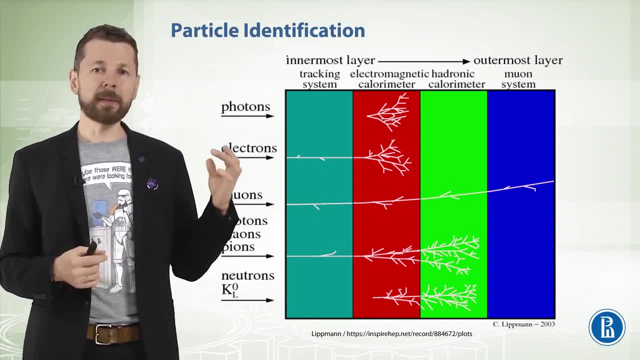 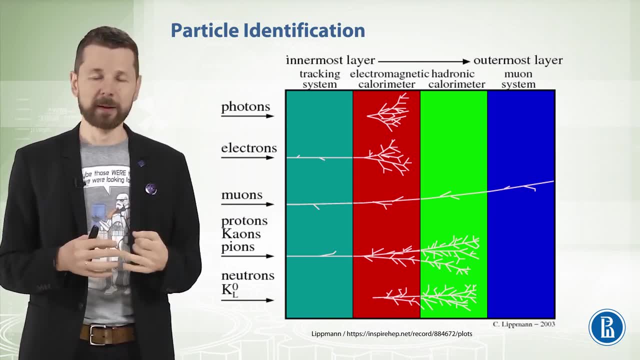 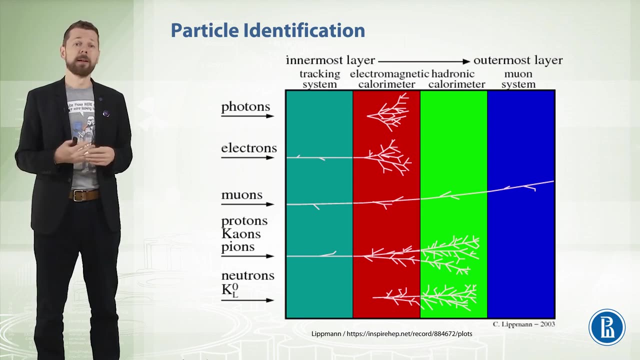 For example, electrons leave tracks at tracking system and electromagnetic colorimeter Photons leave no traces in tracking system but leave traces in electromagnetic colorimeter. Hadrons such as protons, kaons and pions leave tracks in innermost tracking system in electromagnetic colorimeter. 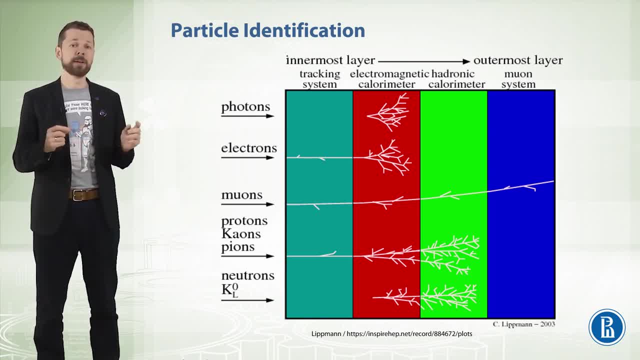 and hadronic colorimeter. And there is a special kind of particles that are called muons. They are heavier brothers of electrons that fly through the whole detector and leave traces everywhere. So collection of the information that those sub-detectors provide allows us to. 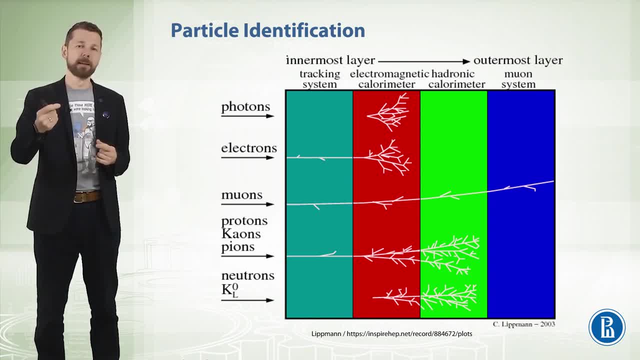 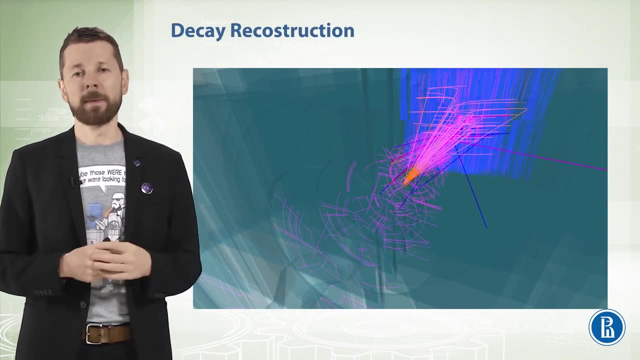 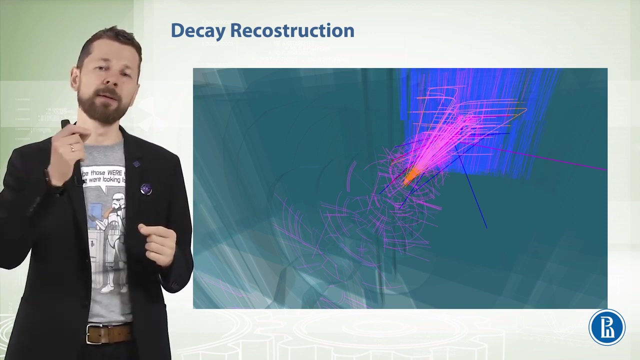 deduce the type of the particle, and this actually is one of the machine learning problems that is being solved at every experiment. After you got the picture of individual tracks, it is important to reconstruct the whole image, the whole event that consists of tracks and vertices. 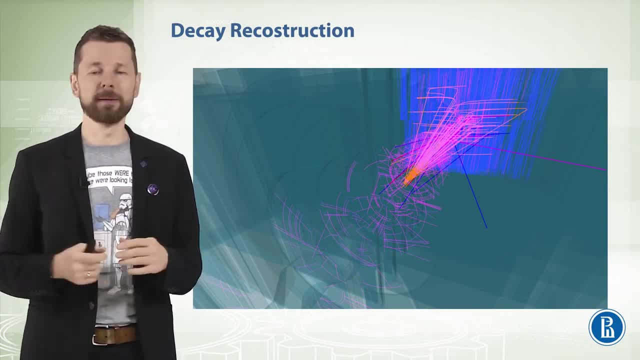 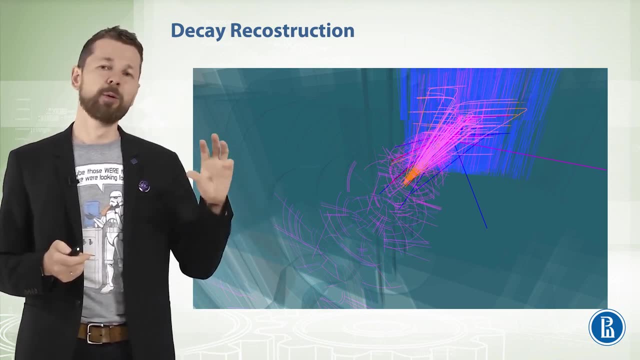 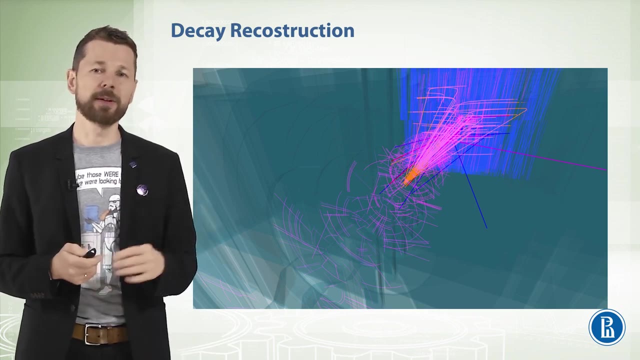 that happen during the particle decays. So on the slide you see just the same collision. that will look from the perspective of vertex locator. So it is exactly the same trajectories And if you look closer you will see that there are secondary 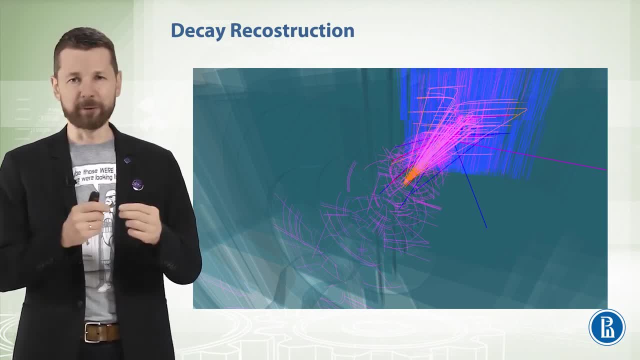 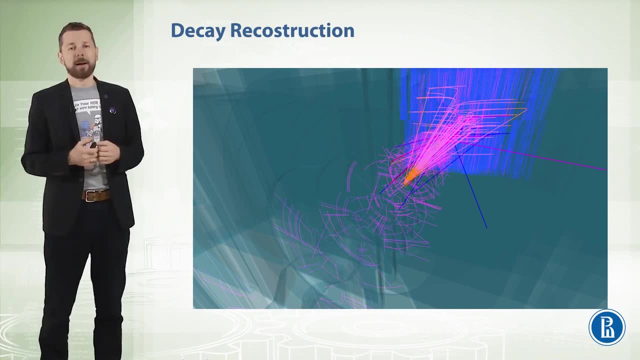 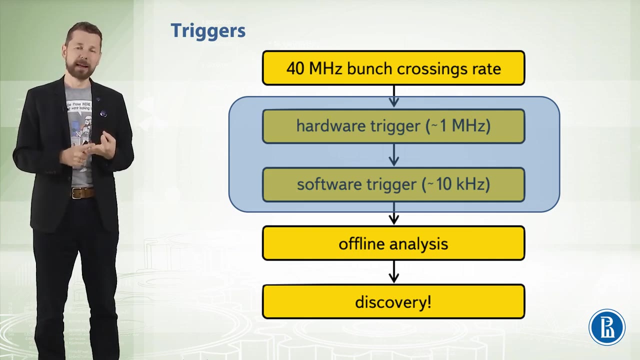 so-called secondary vertices. that correspond to a very short flight of a particle that is then decayed into something else. After these trajectories, particle identification and vertex identification has been happened, we still have to understand whether or not, inside this event, something interesting has actually happened. 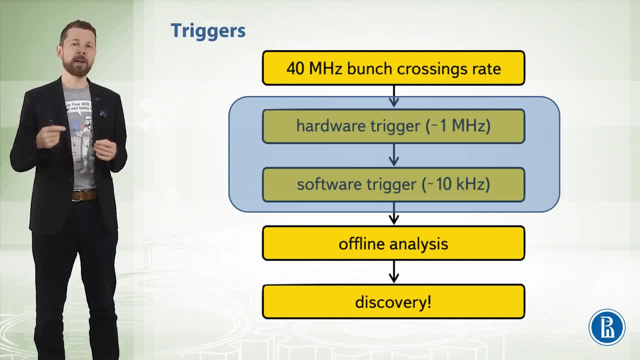 And for this purpose we have a special selection procedures that are called triggers. There are two stages of triggers. The first one is hardware trigger that reduces the rate of the event from 40 MHz to 1 MHz, And there is a software trigger that reduces this rate even further. 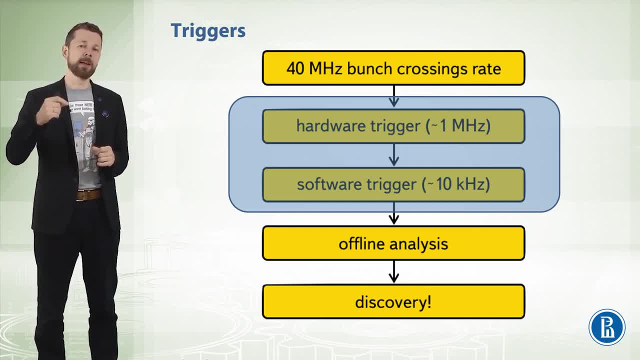 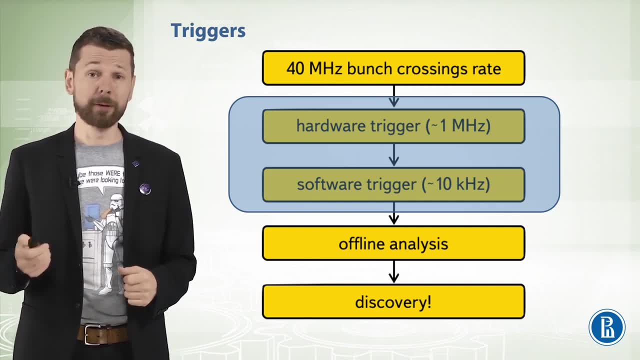 And output of this trigger is being used for offline analysis and eventually for discovery. Design of the triggers is actually quite interesting problem from machine learning perspective. My group has been taking part in design of the triggers for LHCb experiment and it works in data taking since 2015.. 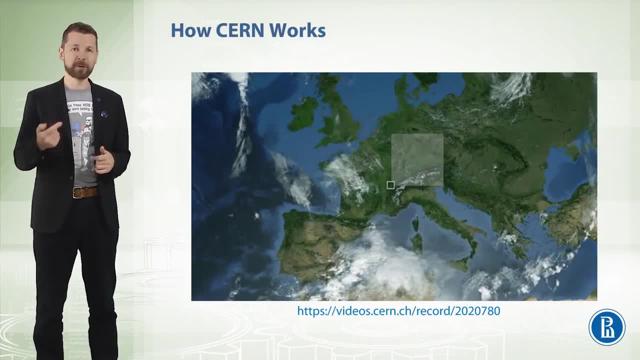 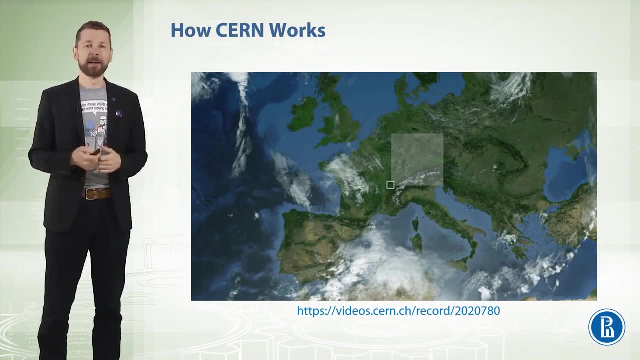 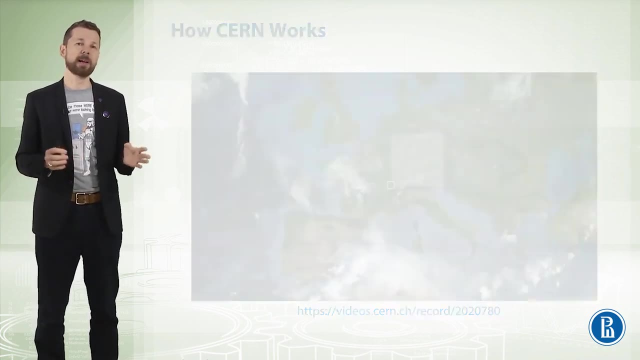 More detailed animation about the design of CERN and how it works. design of LHC and how it works you can find if you follow this link and you see the movie produced by CERN. And at this slide I collected examples of machine learning challenges. 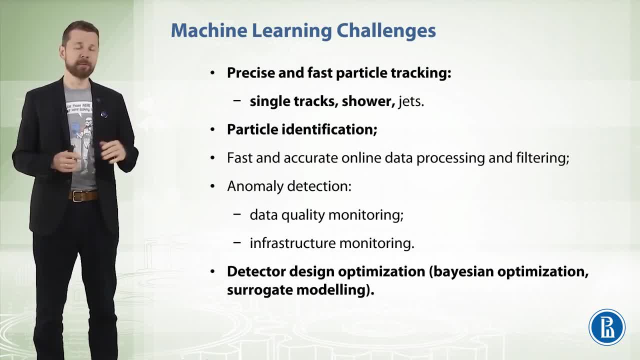 that are related to the topics that I've briefly scratched. So: precise and fast particle tracking. Single tracks, showers and jets- kind of objects that detector operate with Particle identification. How can you discriminate between different kinds of particles? Fast and accurate online data processing. 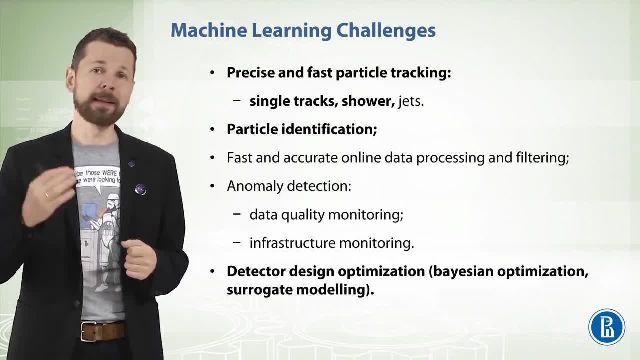 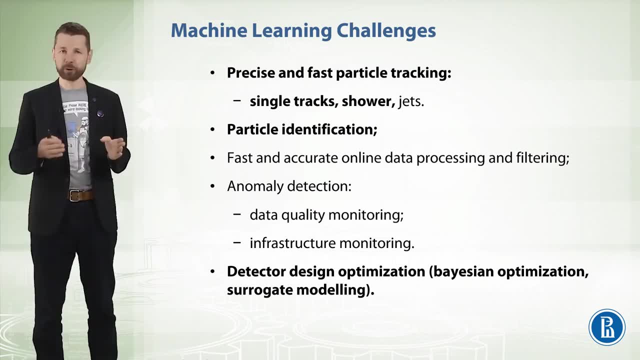 and filtering, How you make sure that the data collected can be trusted. If there is anomaly happening during the data taking- and you should disregard the amount of data taken during the period- you should take certain measures to fix the infrastructure, to improve quality of the data. 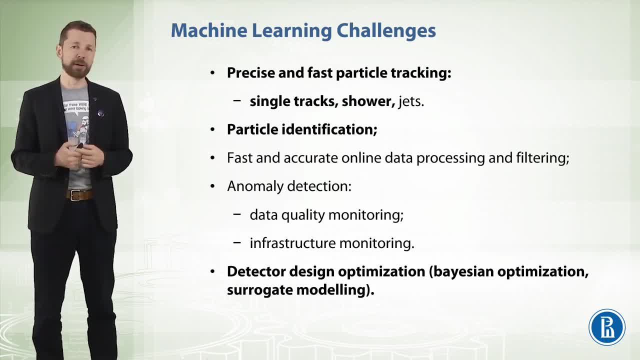 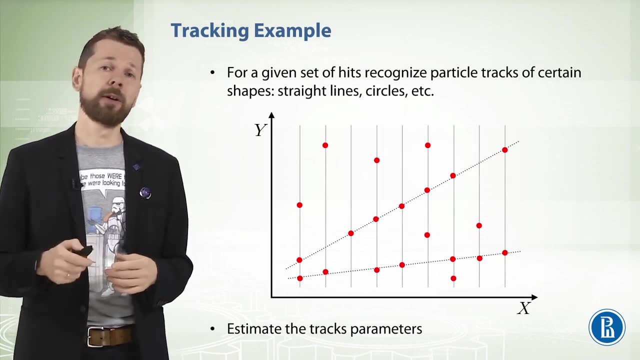 And, of course, the very interesting topic of design optimization of the detector, where various techniques like Bayesian optimization and surrogate modeling can be used. And here's an example of the tracking problem that we'll cover during the next lecture, Given the set of hits represented by points here,